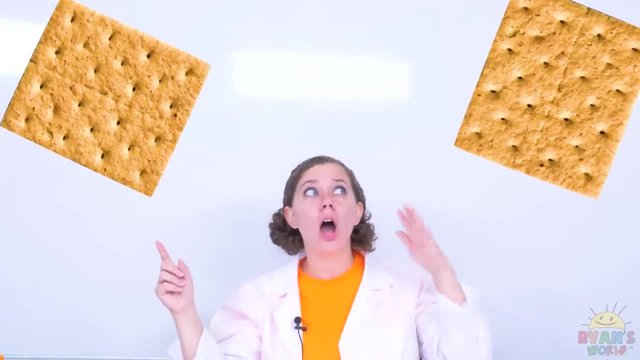 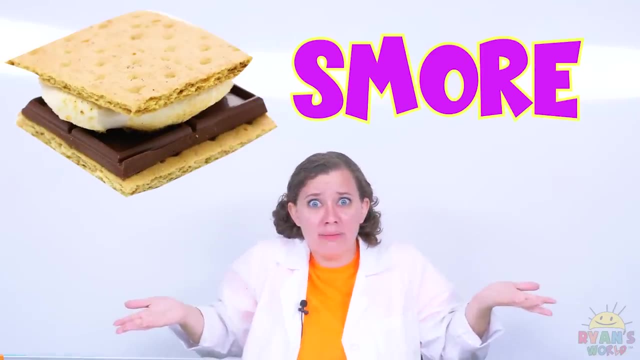 To make a s'more we need graham crackers, chocolate and marshmallows. Then all you have to do is put it together. That's a s'more. Sounds great and all. but where are we gonna find this stuff? 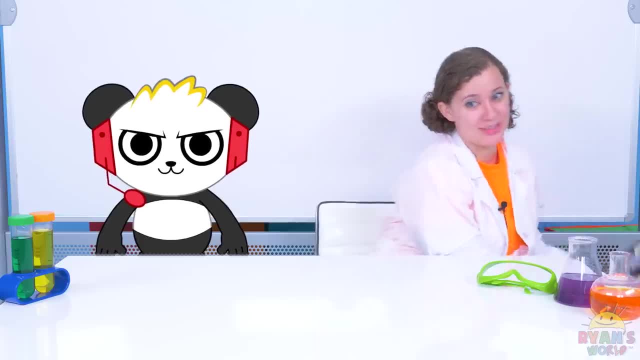 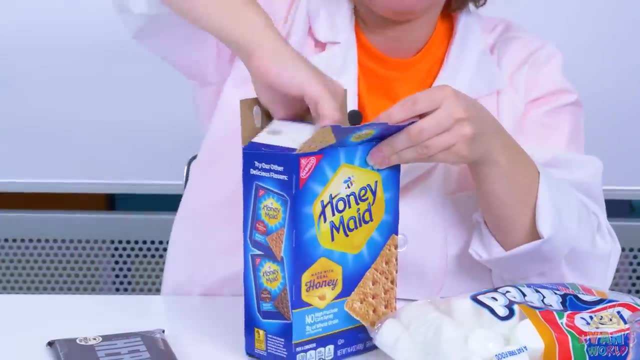 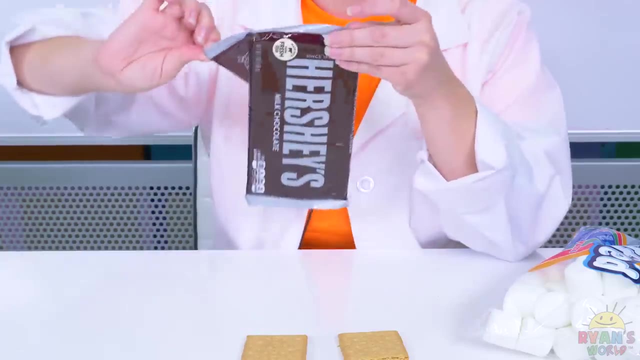 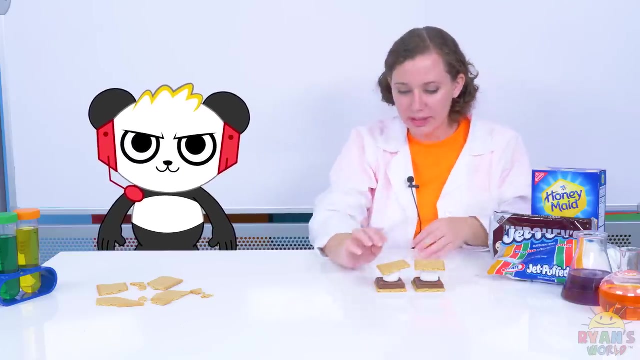 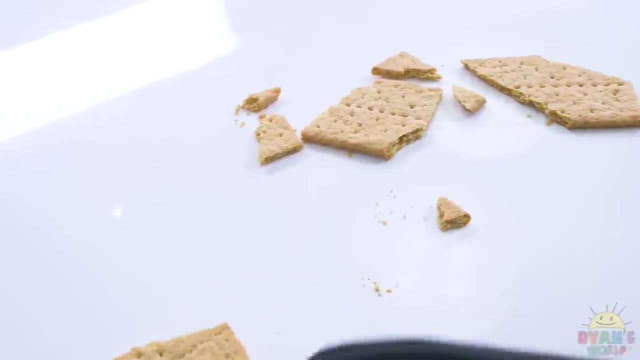 Well, it is about snack time, so I have it all right here. Ewww, Hey Combo, can you help clean up that mess please? Mmm, with pleasure. Ooh, gotta get that piece. Mmm, those graham crackers sure were good. 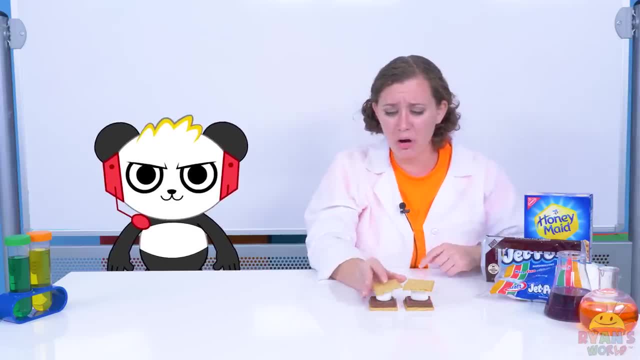 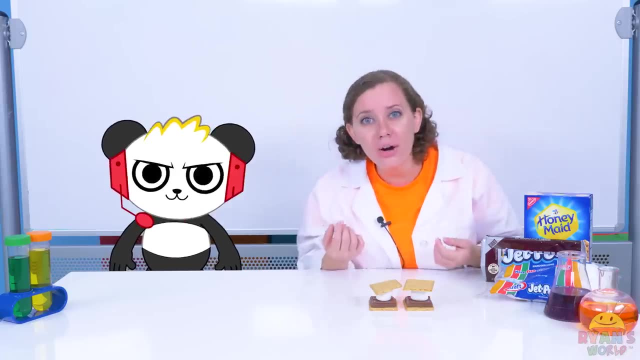 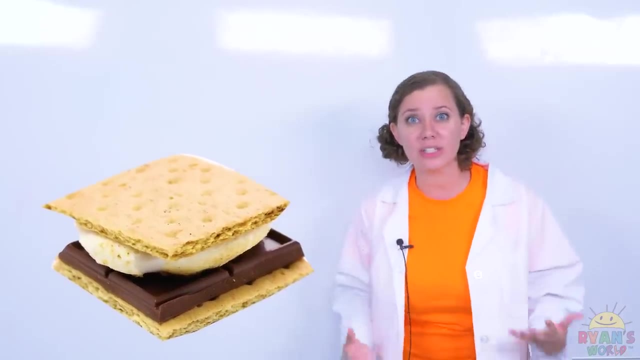 Hey, what's going on with the s'mores? Well, I have them all built, but they don't look right. Uh yeah, they're supposed to be melty and gooey. Oh, I know what we need Now: to heat up the s'more, we need to use a really big heat source like the sun. 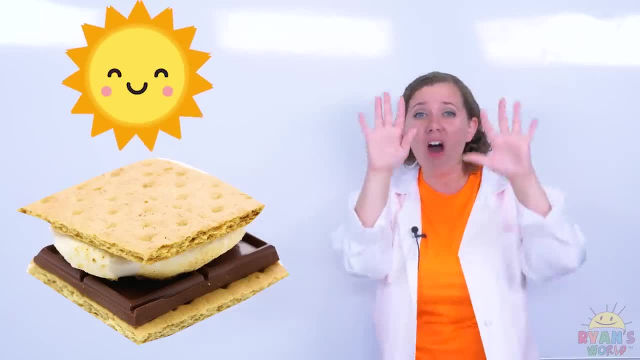 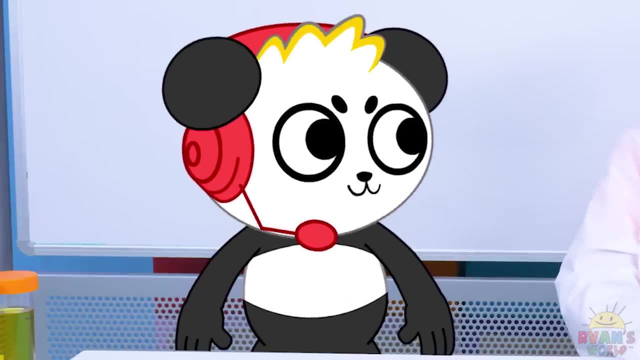 Ooh shh, it's so bright. Now the sun sends down all these sun rays that we can use as solar power to melt the s'more. That sounds cool, but how do we get solar power? Well, that's really easy. All we have to do is use a box to trap all that solar power as heat. 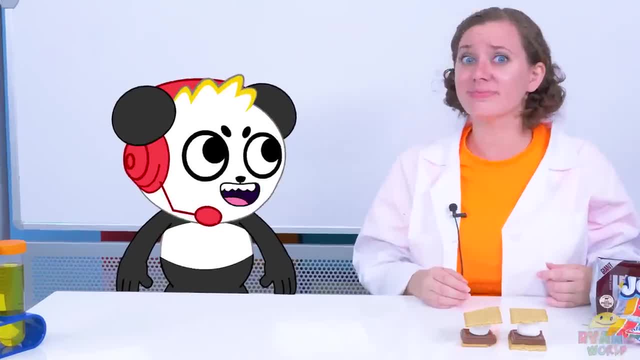 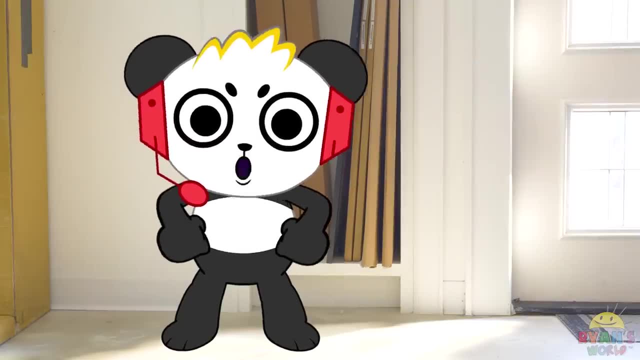 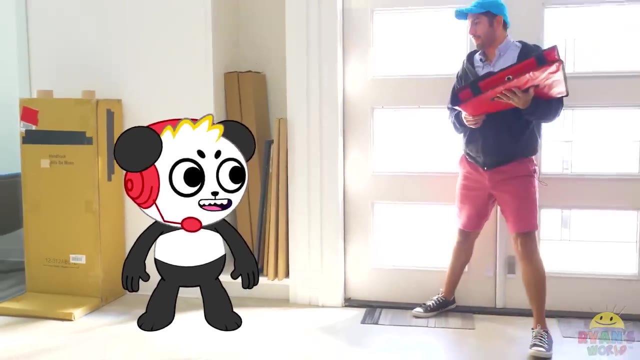 And the best thing is we can just use stuff around the house, Around the house. you say I'm on it, Be right back, Let's see what we can find around here. Are you Combo Panda? Yeah, I'm Combo Panda. Is that pizza for me? 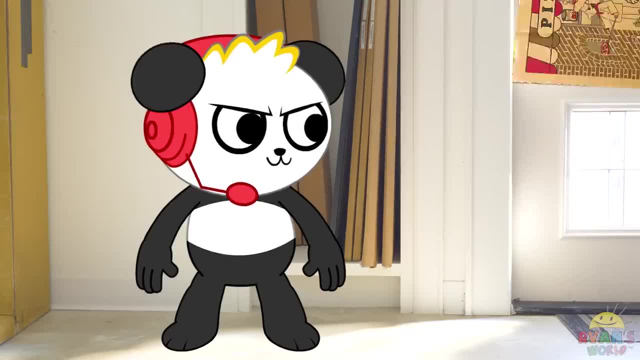 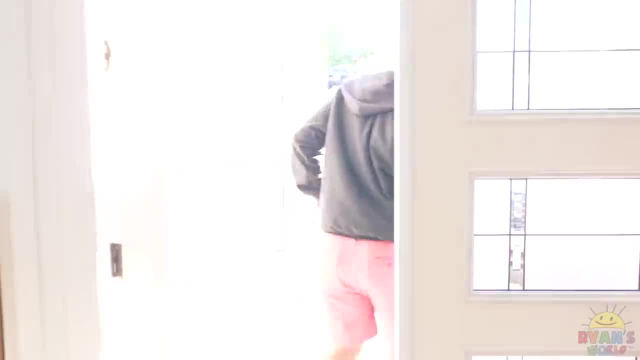 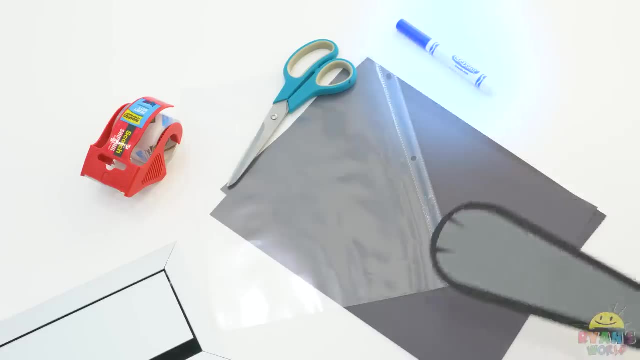 Here you go. Thanks, pizza dude. Anytime, bro, Like your videos, Catch you later. Yeah, I got a pizza all for myself. So here I got some office supplies. I got a marker, some scissors and even some tape. 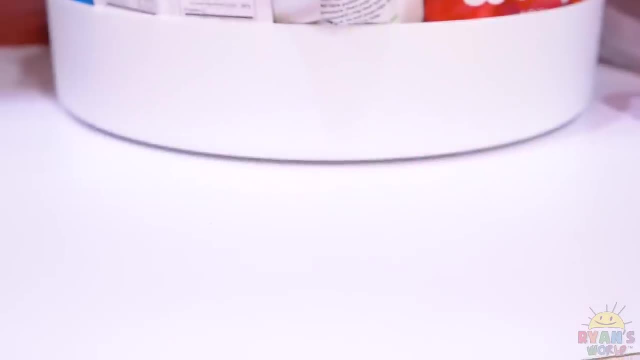 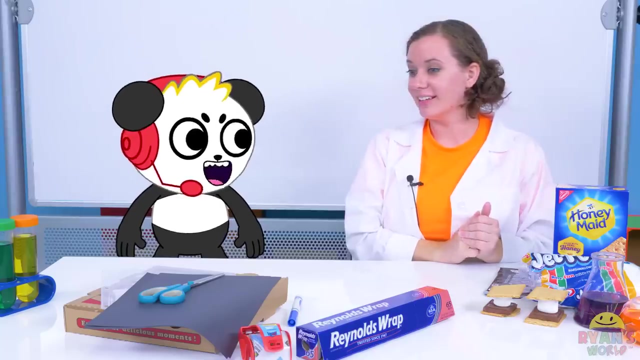 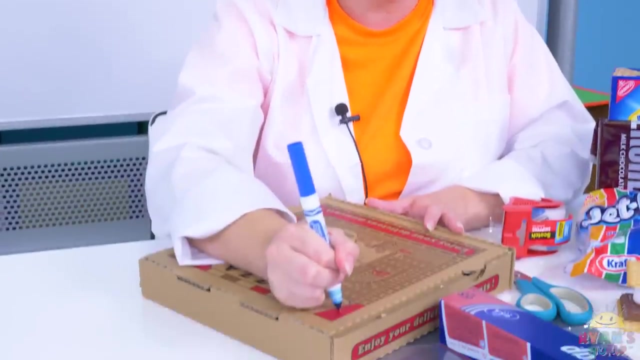 And now we just need some foil. Combo Bunga- Oh hey, Combo, that was really fast, Yeah. and now I've got all the stuff we need to make the oven. So let's get building. So the first thing that we have to do is we need to draw a window for our solar power s'more maker. 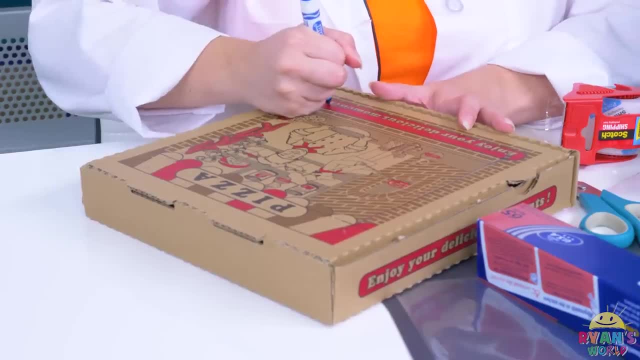 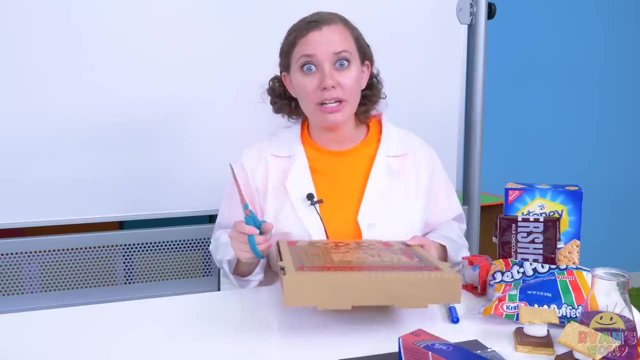 So we're just going to draw a nice big window to help us cook all of those s'mores. Now that we have it drawn, we need to cut it out, This part. make sure you ask an adult for help. okay, Let's see. 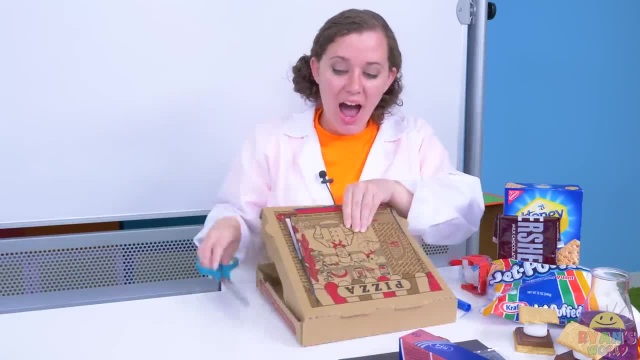 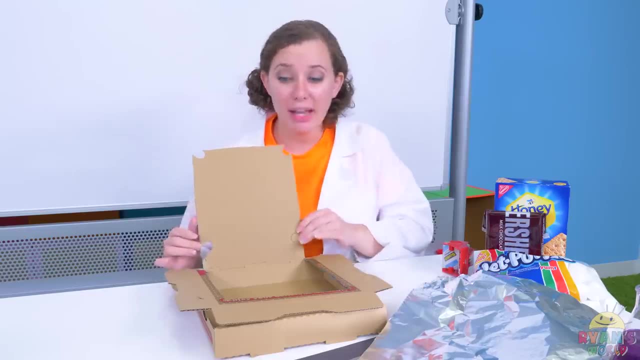 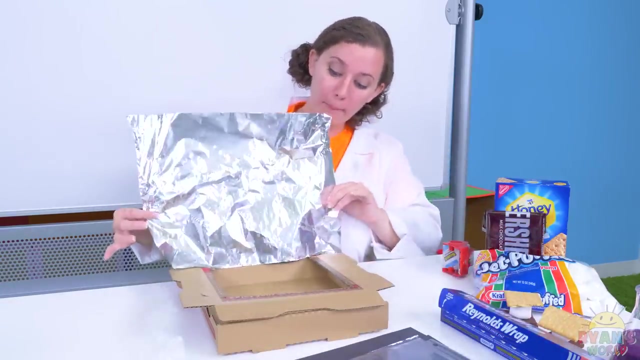 Whoa, Look at that, We have a big window. So next we're going to make a reflector panel to catch all of those sun rays and all of that solar power by using aluminum foil. Shiny Alright, that looks great. 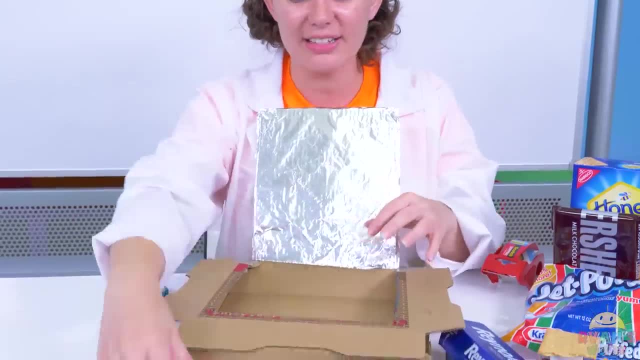 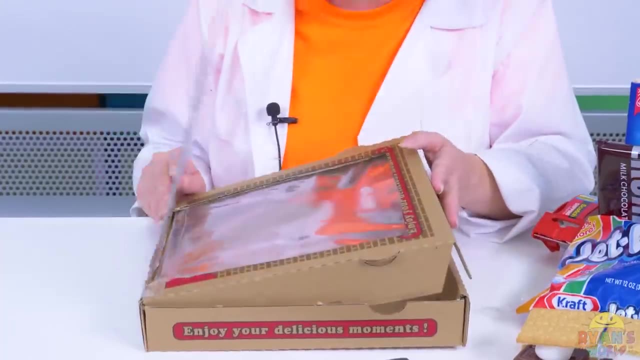 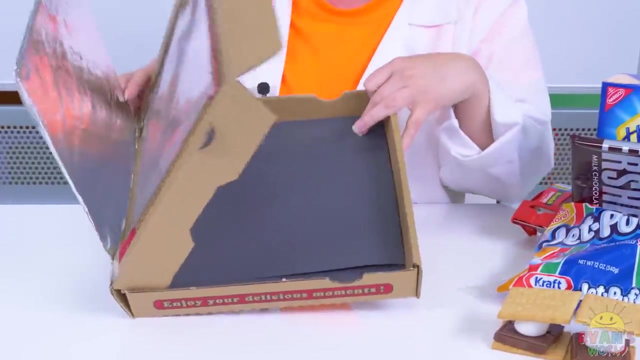 Now the next thing we need to do is chop in all the heat. So we're going to use this piece of plastic Just like that. Like that- Ooh, alright, That is nice and steeled. So the last thing that we need to do is just put the black paper in to help us absorb all that heat. 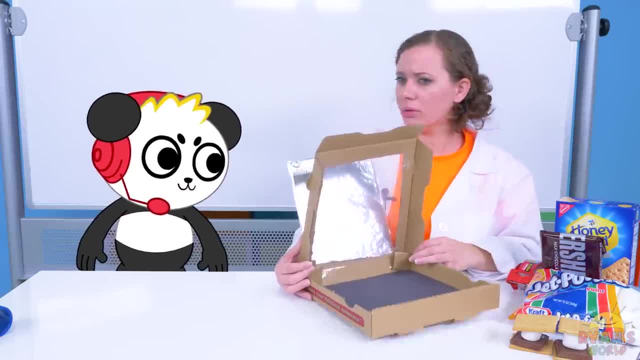 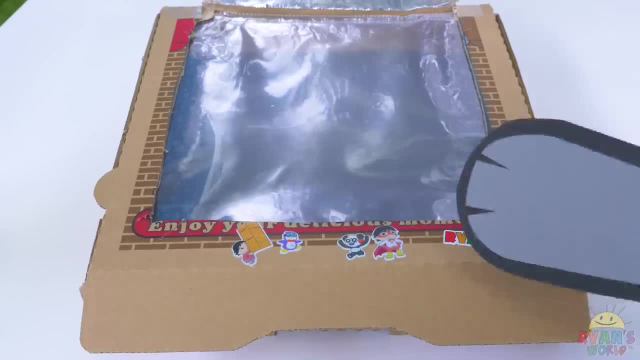 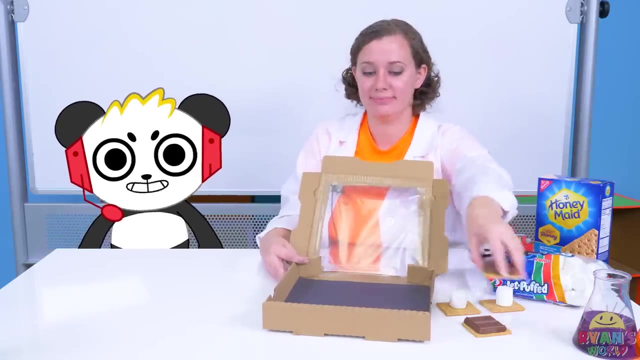 And done. Hey, we're not done yet. What do you mean? It looks done. I could use one more thing, And there we go. Oh yeah, Some Ryan stickers on there Looking good. So now we can just put the s'mores in and we'll take them outside and see what happens. 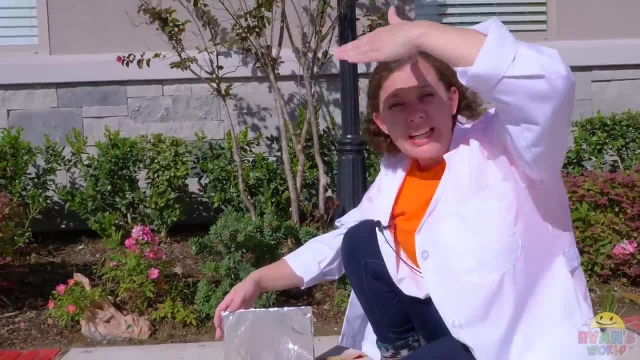 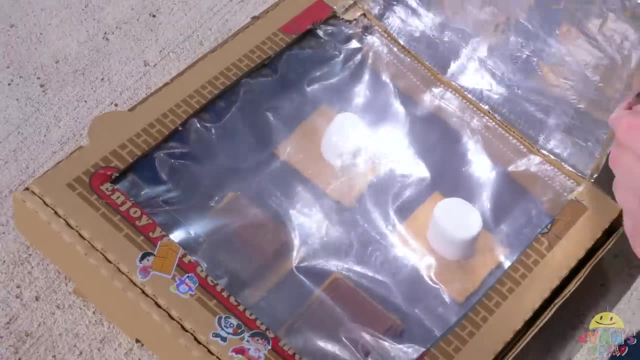 So, as you can see, it's really bright outside. Now we're going to use all of the sunlight to cook our s'mores. Now we just have to adjust this panel to get it just right. Ooh, that looks really good, right there. 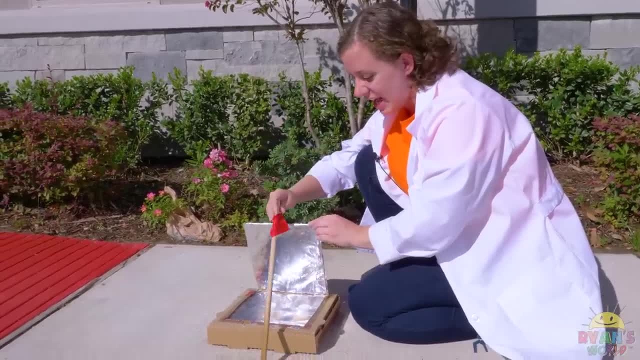 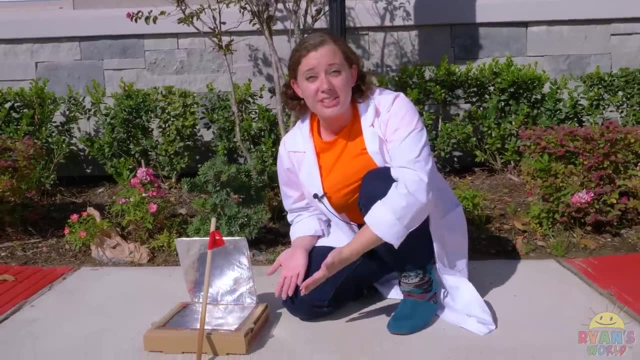 Now we can hold it in place with a stick. I put a little bit of tape to tape it right in place. All we have to do now is just wait for the s'mores to melt, And then Combo can deliver them to Ryan. 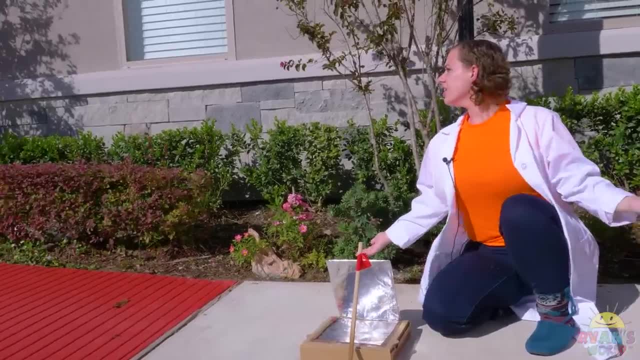 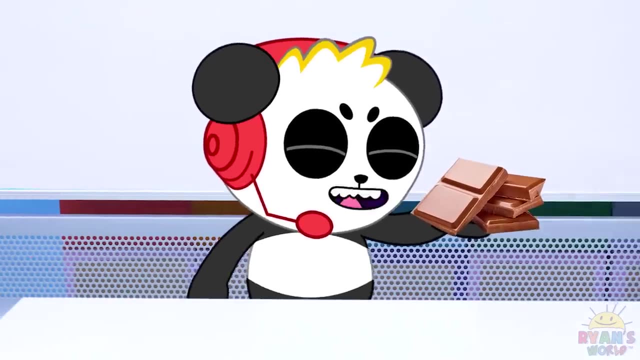 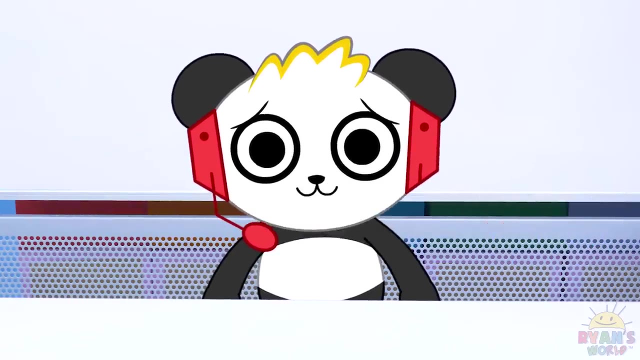 Wait a second. Where is Combo, Combo, Mmm. this chocolate chair is yummy Combo, Uh-oh. Oh, Ryan's s'mores probably ready by now. Yay, One hour later. All right, Bray, let's check out our results.